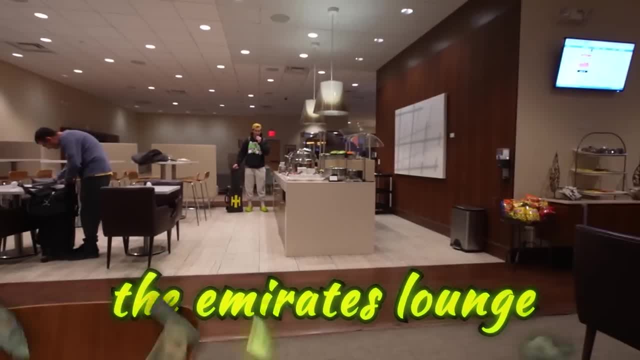 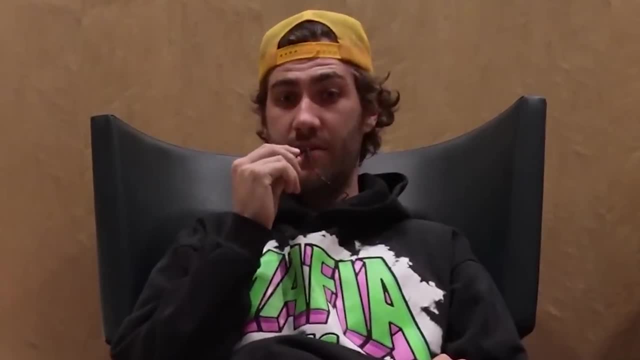 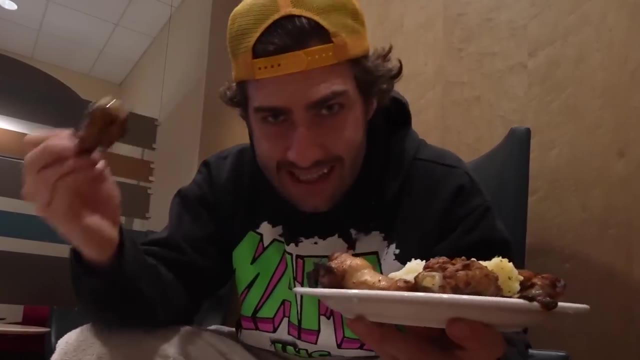 needed to get on the plane, So I decided to check out the Emirates Lounge. This place is huge. It's just me and all of this food. This is a service that comes included with your ticket. Welcome to the Emirates Lounge. We have chicken wings, mashed potatoes, coffee and cubed cheese. I'm going to squeeze every last. 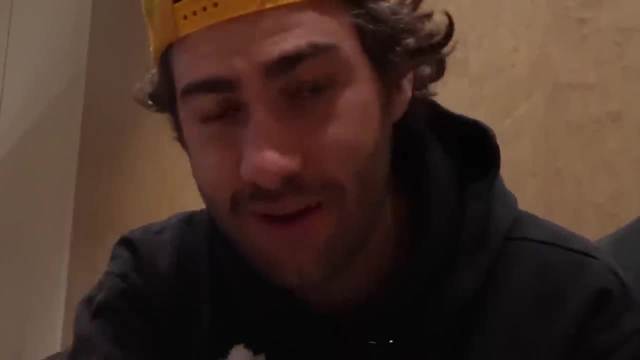 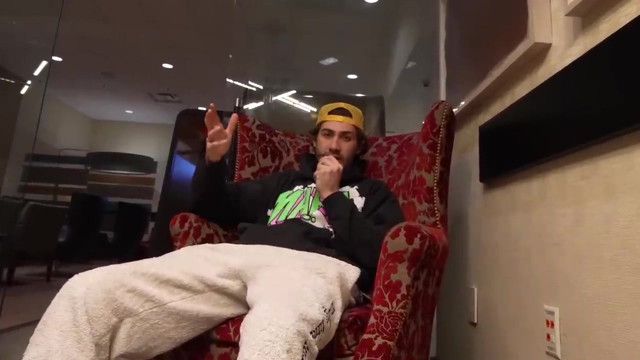 drop of luxury out of this experience possible, and I'm going to bring you guys along the way. The privacy inside this lounge is actually crazy. If you ever go into a lounge inside of an airport, they're normally packed full of people. There's like a line. 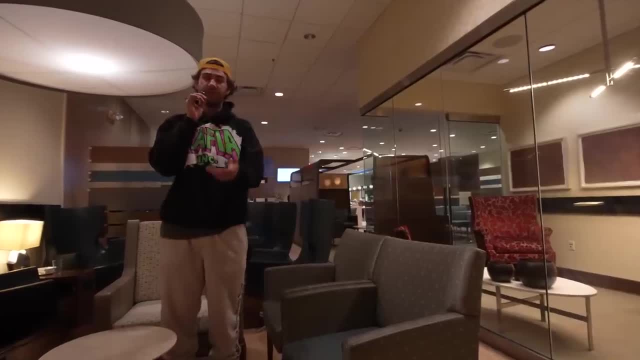 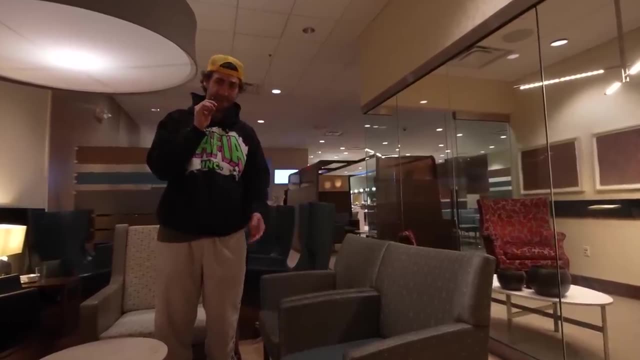 Outside. this place is silent. Sometimes when I'm traveling, I'll pay to go into a lounge to take a shower, which is a game changer if you have never done that. The Emirates Lounge does not have showers, but I hear there's a shower in my suite. Tell this guy to stop yapping and just show me the. 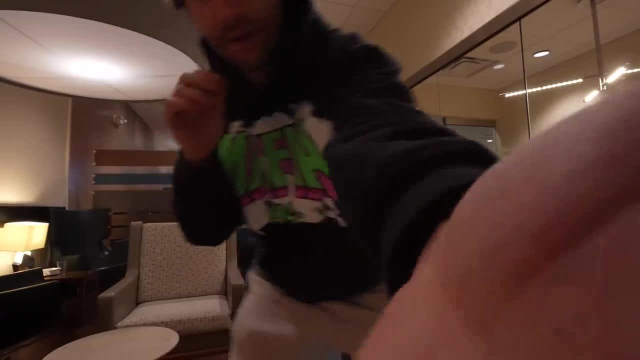 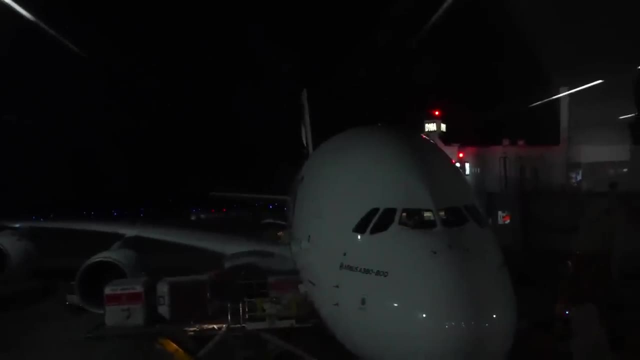 cool plane seat. huh, The flight does board in like five minutes, so we have to go. The line to this plane right here is huge, and that's because this plane right here that we're about to get inside of is the world's largest passenger plane. It's two stories tall. I'm not going to be able to. 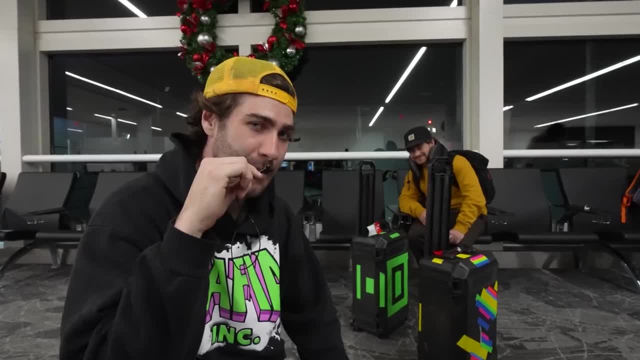 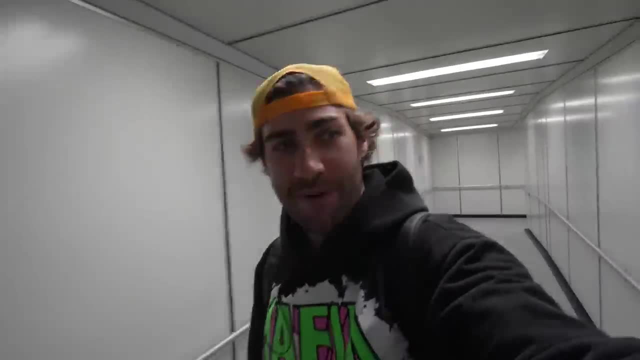 actually never been on one of these before and it is massive. Let's go on that plane, huh, All right, Thanks so much, Here we go. I've waited years for this moment and now, today, I experience it for myself, mainly thanks to you guys. Thank you for subscribing. That's why 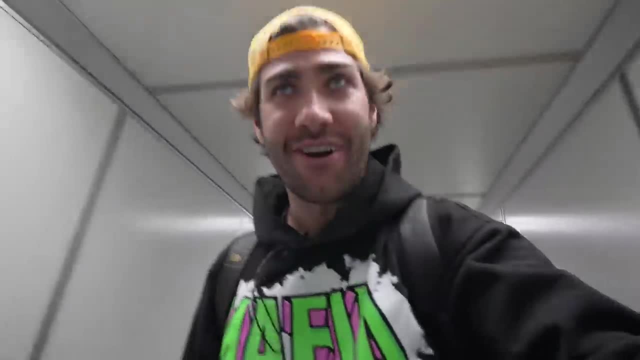 Emirates gave me this seat and now we're going to experience it together. I don't know what Eric's doing, but I'm having a great time. That guy's a freaking idiot. I'm sitting on the floor eating my chips and I'm having the best day of my life. 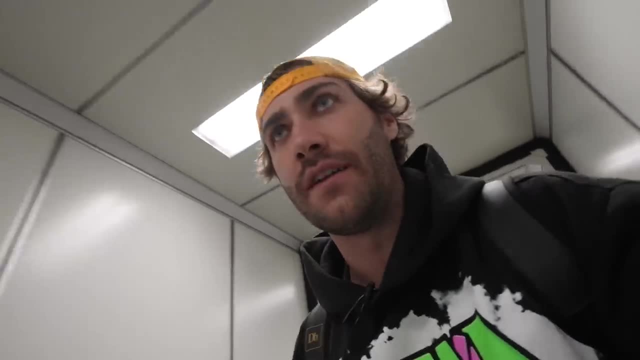 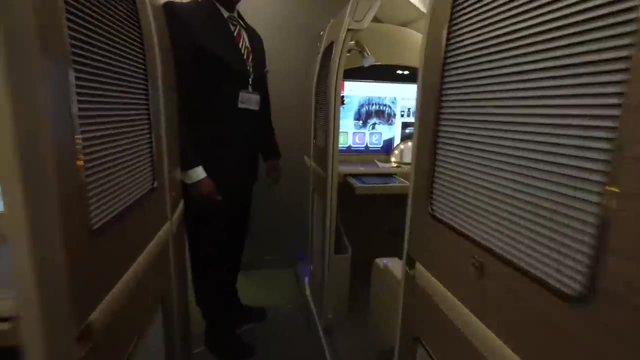 If you guys don't know, on my Instagram I always do a gap check on airplanes. I'm always afraid of falling through the gap, so let's do a gap check here. Nice gap, though This was insane to me. The first class section takes up almost the entire top level. 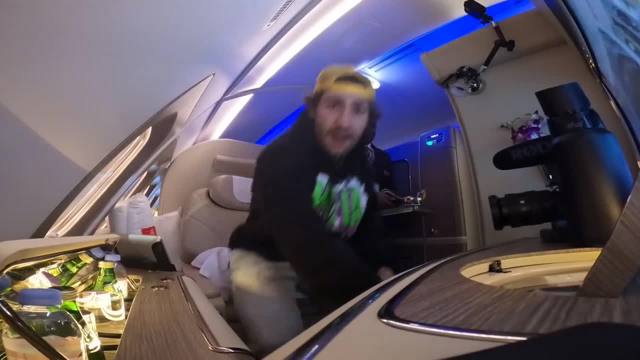 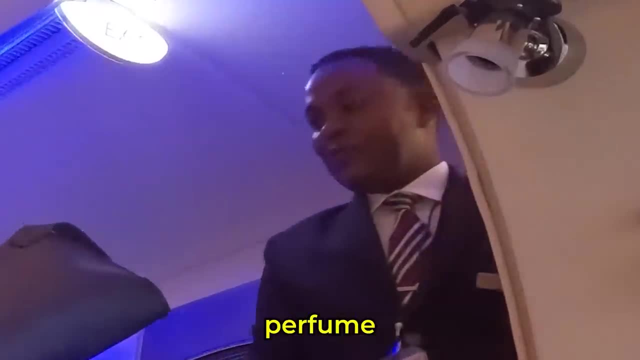 Every single seat is like its own little house. Thank you, David, Appreciate you All right. What are we looking at here, David? And that's your kit bag, Kit bag. What's in here? Toothbrush, shaver, perfume. 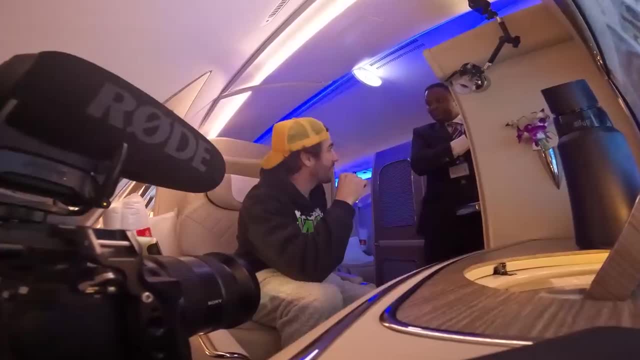 You guys thought of it all. There's a spa, also Spa, And a shower. Oh my gosh, You're going to take a slot whichever time you want to take a shower. I love it. This is the writing card and a pen. 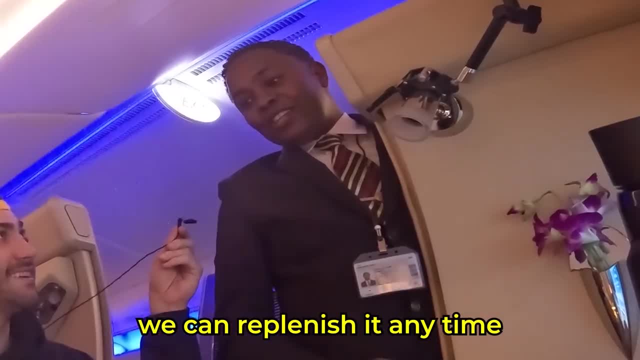 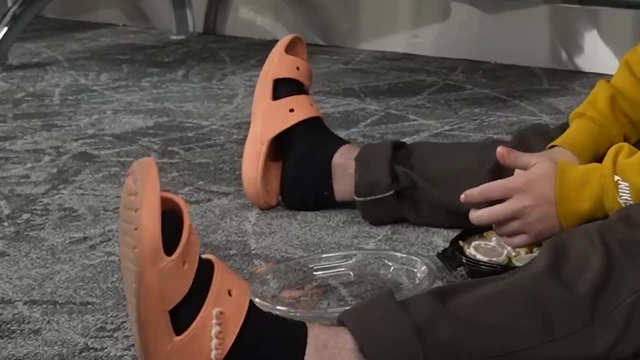 A mini bar. A mini bar- Yes, I like this. You can replenish it anytime. This is like a hotel room, where you pay for what you drink or everything is just free. I'm so freaking out. That's crazy. Yeah, the floor is dirty, but so am I. 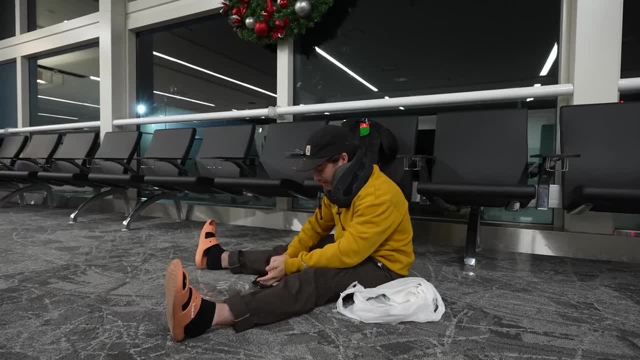 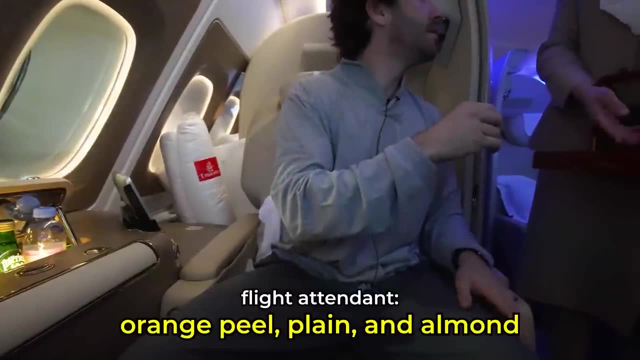 And I'm not afraid to admit that I'm like Eric, a freaking idiot. He's probably eating caviar and having his freaking toenails clipped right now. Would you like to have some dates? We have some dates with Orange, Peel Plain and. 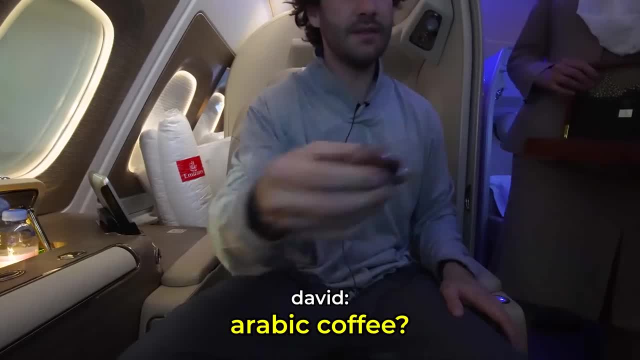 Let's do Plain. Is that this one? Yeah, Great, Thank you so much. That's awesome. Arabic coffee, Arabic coffee. yes, Thank you so much. Appreciate that. This place is a never-ending supply of food. Maybe a free towel. 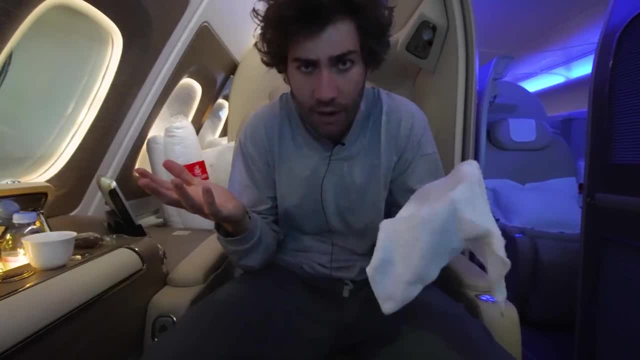 Towel would be amazing. Just never-ending stuff. What do I need a hot towel for? What do I do with this? The craziest part about all this is we are just scraping the surface. We haven't even left the airport. 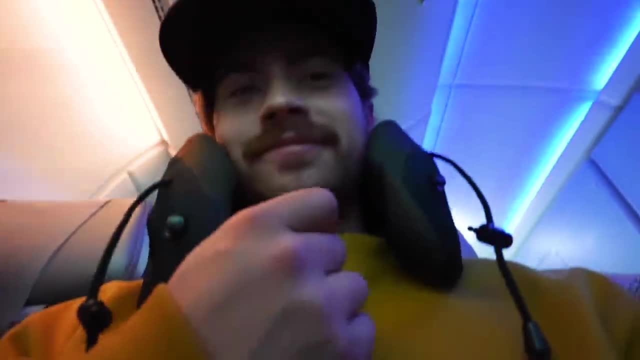 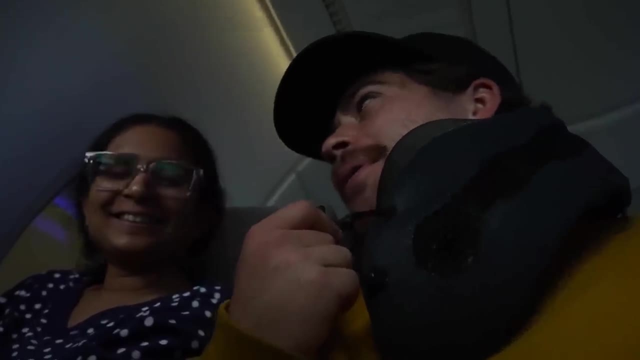 Beans did finally manage to meander onto the plane, Even made a new friend in the process. I'm here with my new friend, Alpa Hi. We're enjoying the benefits of economy. We don't need a shower on the plane or any fancy food or anything like that. 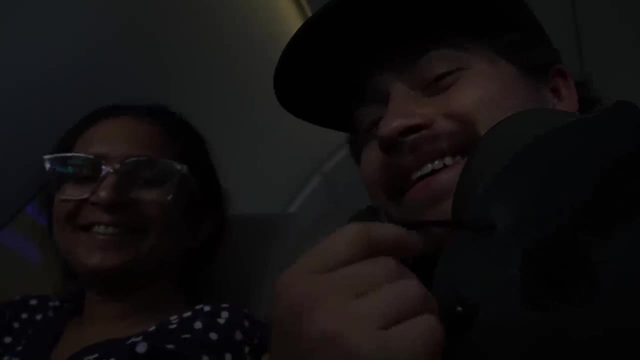 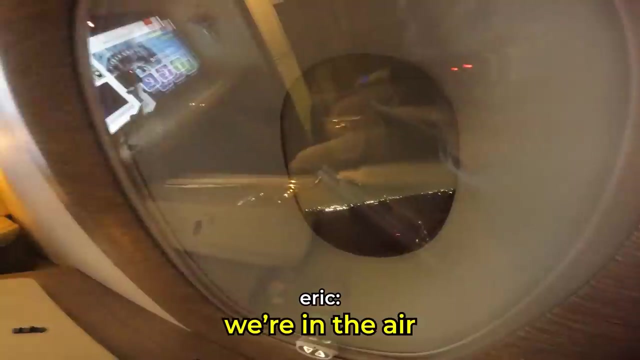 We have the power of friendship. Yes, I agree, I'm a little overwhelmed right now, So I'm just going to sit here and wait for this plane to take off And then we'll do a little tour. We're taking off. 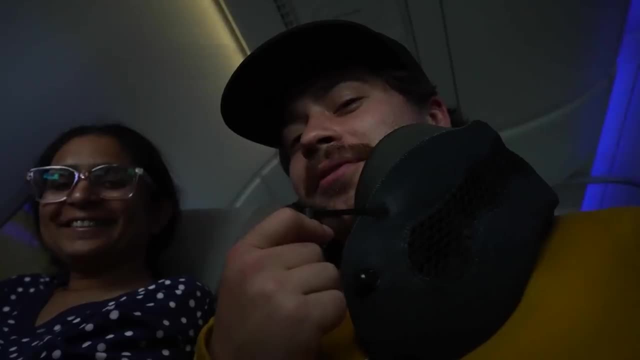 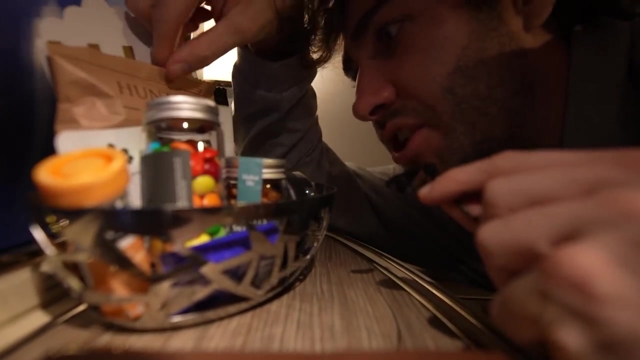 The babies have stopped crying. Eric's probably eating like filet mignon or something right now. It was time to try out every feature this suite has to offer: Vanity Gourmet snack basket with M&M's chips, chocolate. You've got not one, not two, but three touchscreens. 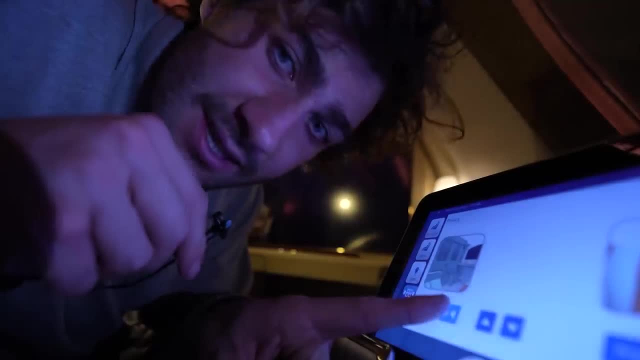 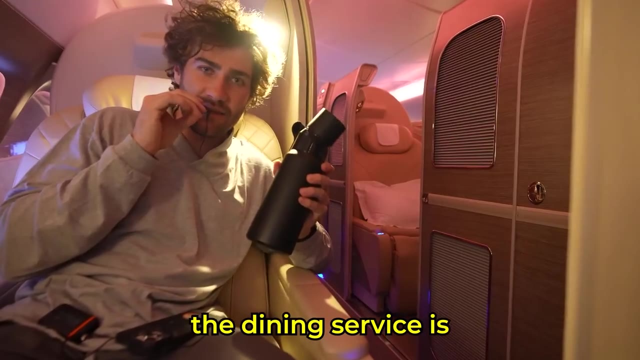 Just press this and my whole seat starts laying down. I press this, the doors start closing behind me. It's basically like I'm flying the plane. Please don't trust me to fly planes. The dining service is whatever you want. There's no breakfast or lunch or dinner or dessert. 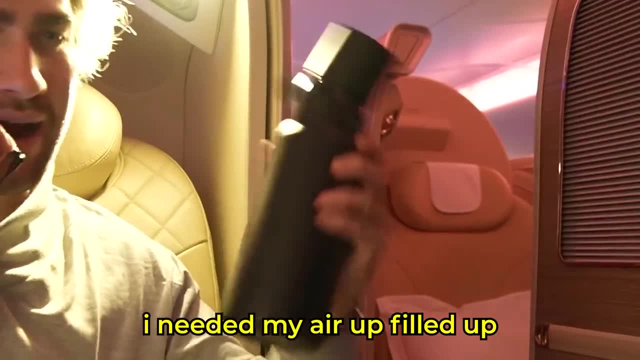 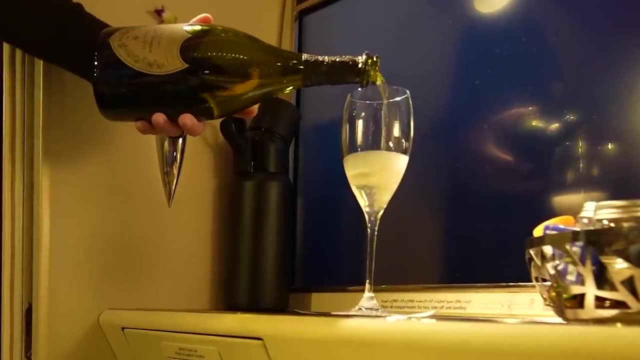 You just ask for whatever you want and they go make it for you in the kitchen. When I need my air up filled up, they filled it up. You understand the freedom in this. It's room service, a private chef and an assistant all in one. 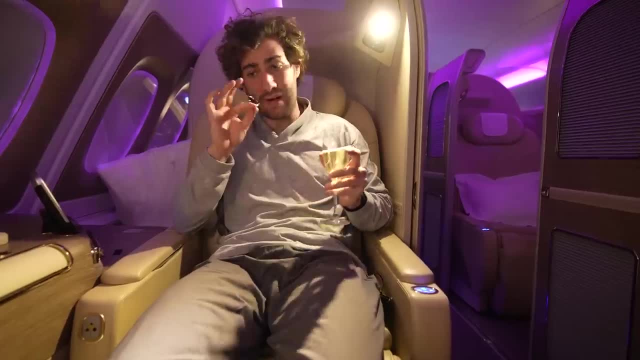 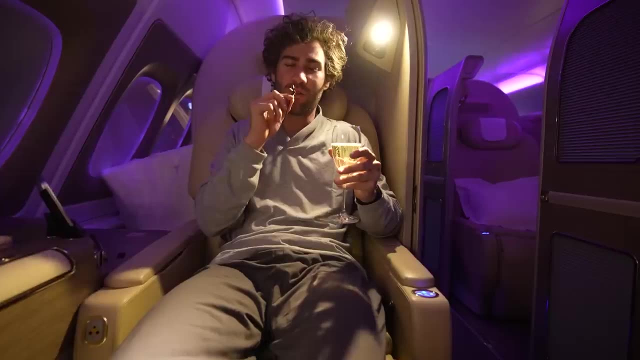 Dom Perignon, probably like a hundred dollar glass of champagne right there. The craziest part about this seat so far to me is the space right over to my left. That is suite 1F, which was supposed to be B1F. 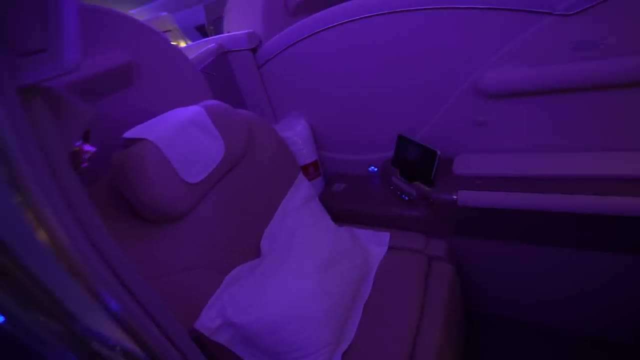 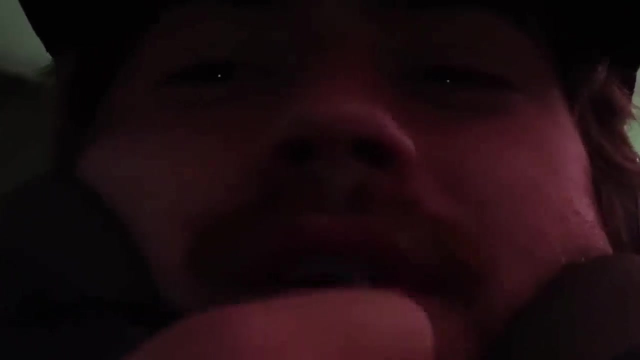 Bean's seat. We literally had the ticket for that seat right there It is completely empty. My man passed all of this up to sit in economy Watching Inception- probably going to watch a lot of movies. Eric's probably like watching some movie on like a flat screen TV. 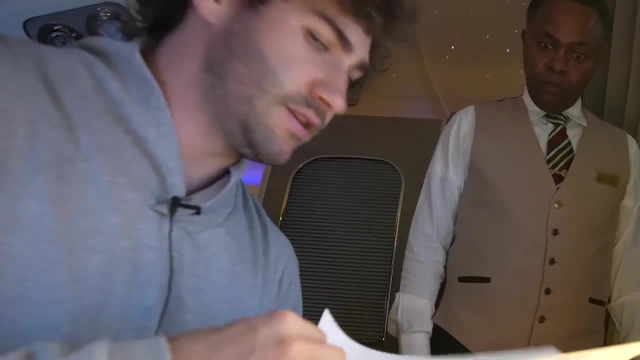 Could I get the popcorn and then the beef sliders? Should I do caviar? Yeah, It's our signature offering. Okay, I have to do it. You have to do it. Okay, caviar as well. Thank you so much. 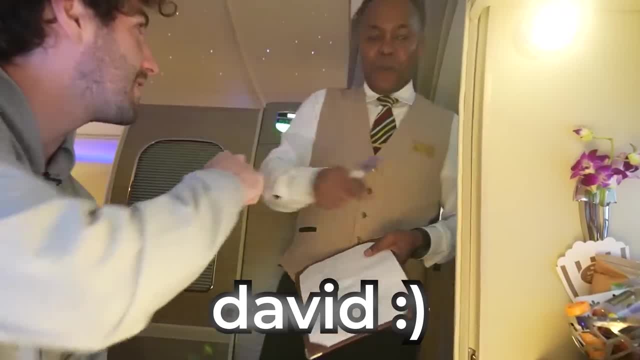 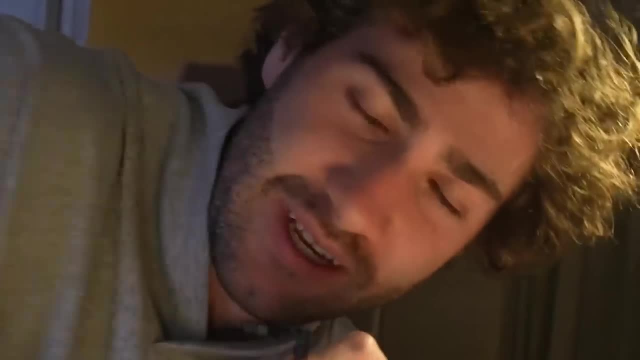 You're welcome. Thank you, David, They're so cool. David and Joe- Oh sweet. And yes, I said two people's names because I have not one but two flight attendants dedicated to this suite. I have the craziest imposter syndrome right now because I'm not this guy. 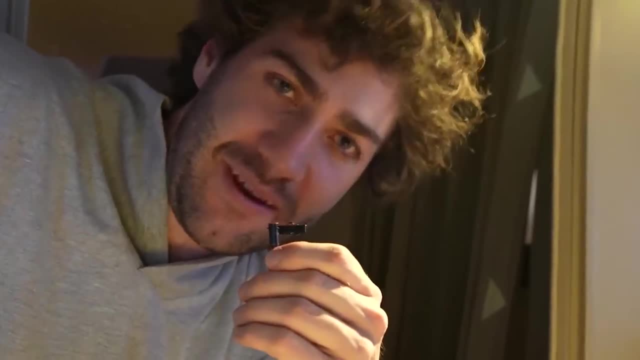 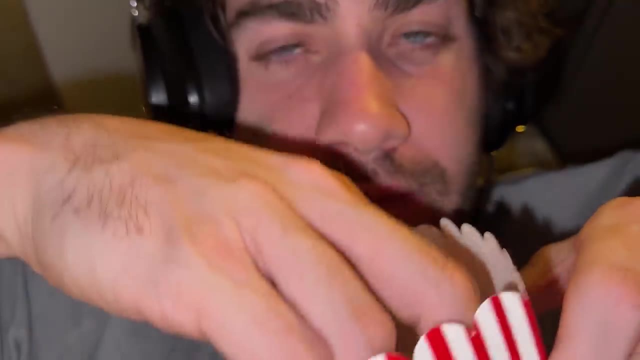 They think I'm the CEO of some Fortune 500 company, but I'm not going to stop them because we made an agreement: Squeeze every drop of luxury out of this experience and share it with you guys. It had been an insanely long 24 hours of travel and I was beyond exhausted by the end of it. 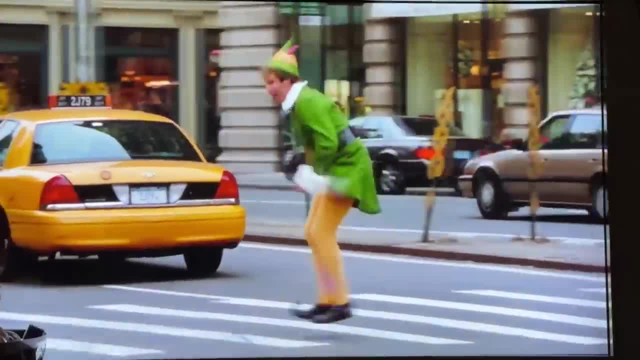 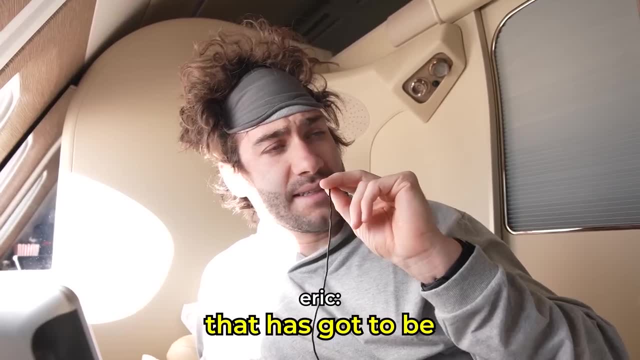 My only goal: use my private flat screen TV to watch Elf, but I was so beat that I passed out within the first few minutes. Good morning Guys. I accidentally fell asleep watching Elf. That has got to be the deepest sleep I have ever gotten on an airplane. 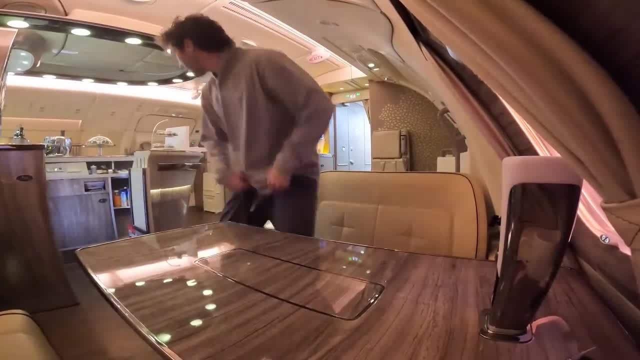 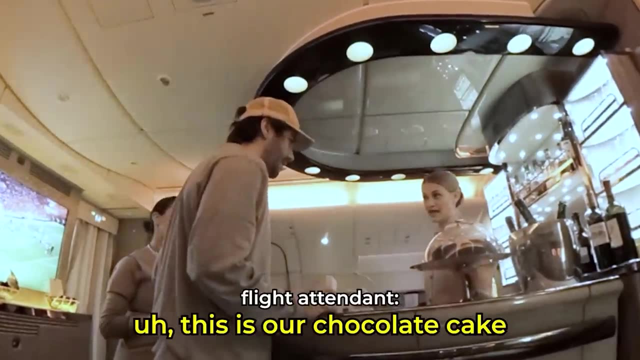 I really did not want to get out. I managed to drag myself out of that super comfortable bed and give myself a tour of the rest of the first class cabin that I hadn't seen yet. What type of cake is this? I guess this is a chocolate cake. 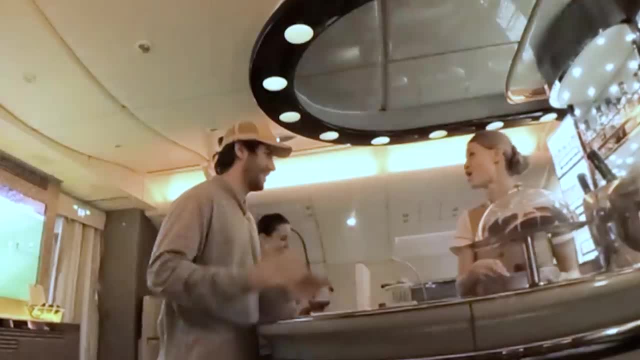 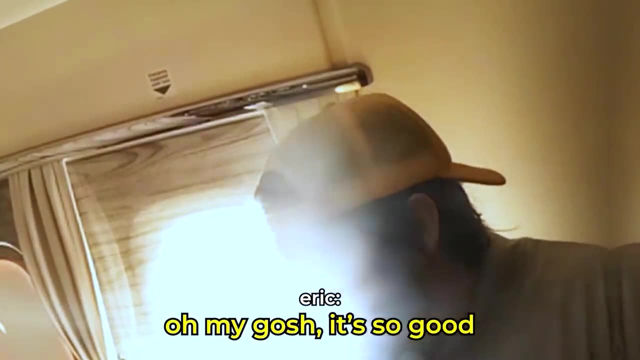 You realize this is like ridiculous, right, It's like a flying car Like this is crazy. Can I just get a regular coffee with cream? Thank you so much. You're welcome. Oh my gosh, it's so good. I hadn't heard from Beans or Howie. 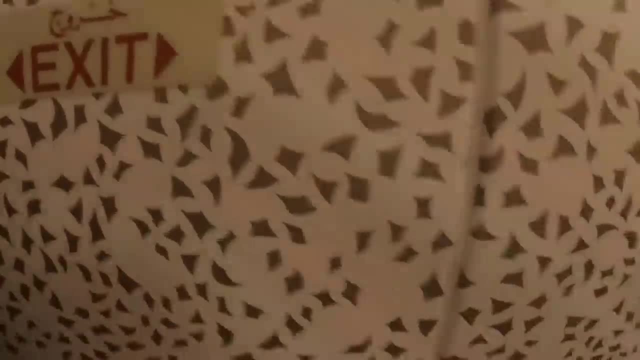 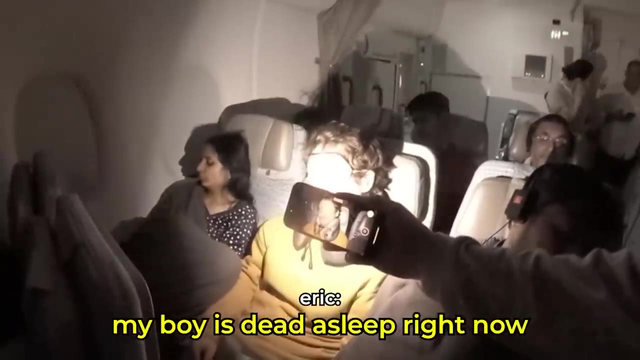 Fortunately, that cake and coffee gave me the energy I needed to make a long voyage down to economy. Beans is in here somewhere. Where's this kid at? My boy is dead asleep right now. I decided to let Beans sleep and headed back to my seat. 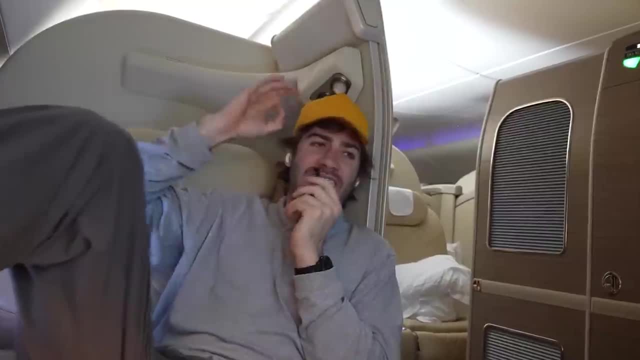 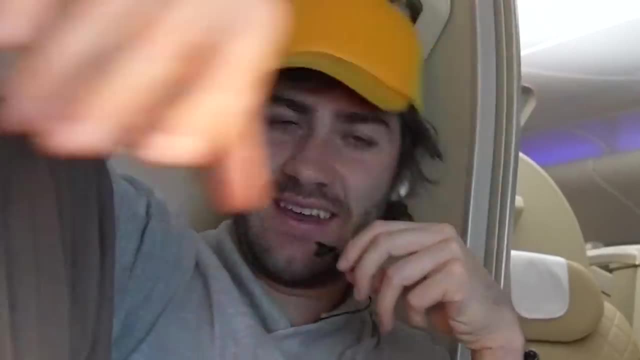 to find out what a full meal on this plane looks like. The power of infinite room service. With great power comes great responsibility, And my responsibility is to order everything And I'm going to gorge myself until I'm sick. By then Beans had managed to get me to the plane. 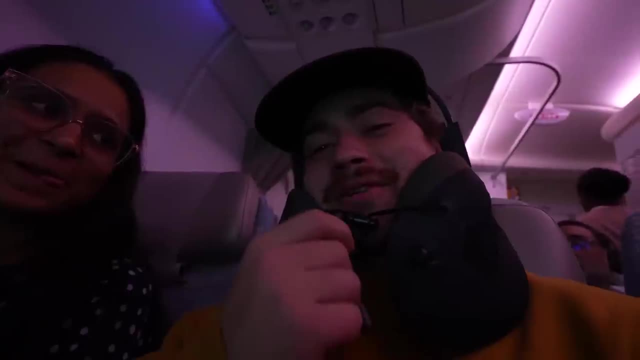 I was like, oh my gosh, I'm going to be sick, I'm going to be sick, I'm going to be sick. He managed to wake himself up in time to eat his own meal down in economy. We're having a great time. 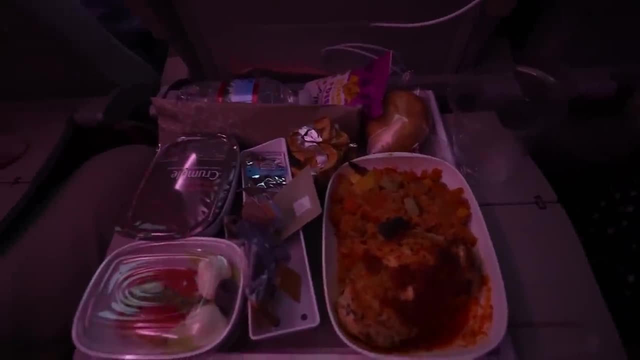 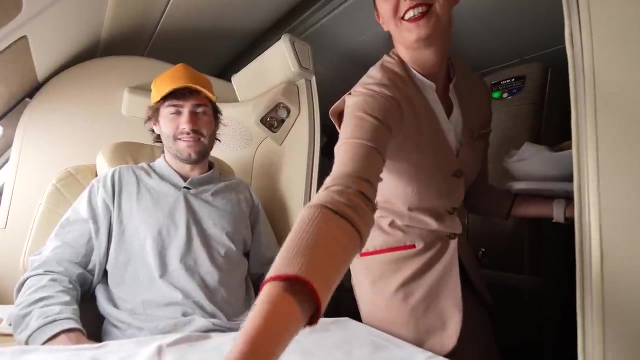 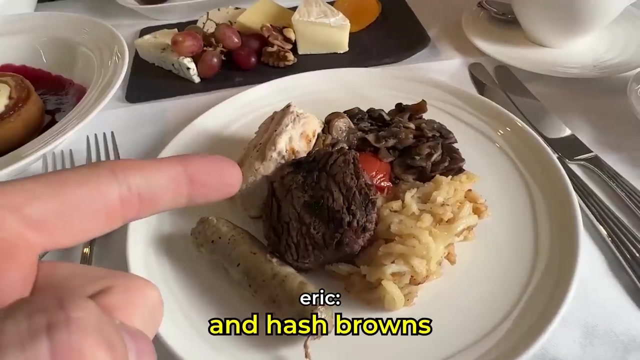 We got dinner rolls. There's some strange assortment of vegetables. It's so delicious. Stay tuned, because things are going well in economy. That looks awesome. Oh, This is insane. We got breakfast meats and hash browns, an espresso, a smoothie. 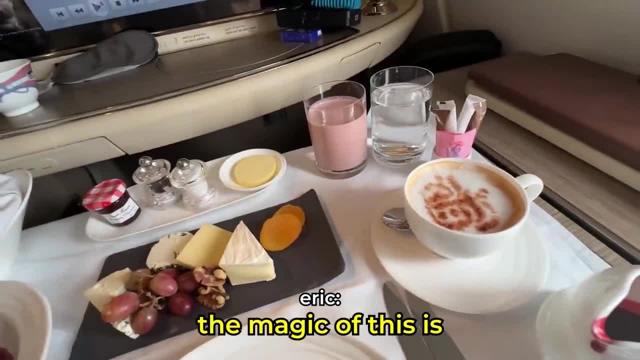 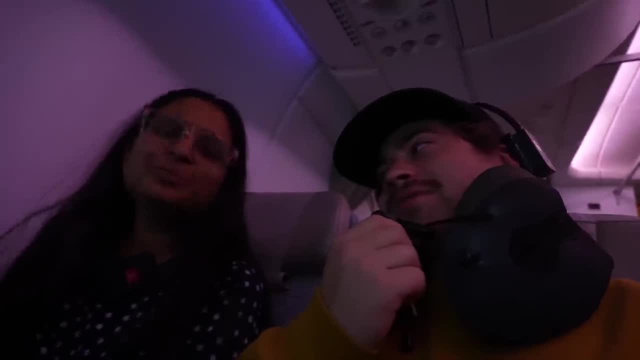 cheese platter, the blueberry torte and bread. The magic of this is I could order this five times over. Eric is probably eating caviar, drinking the finest wine in the world. It goes without saying that this was the best meal I've ever had on an airplane. 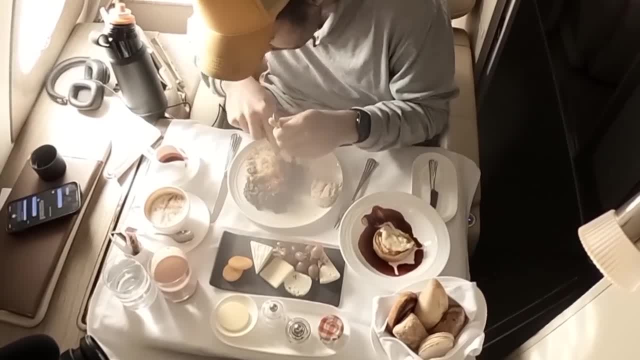 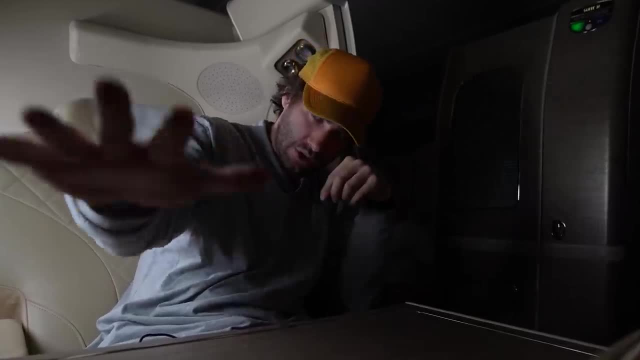 It might have been the best meal I've ever had on the ground, But there was still one more very important thing that I needed to do before this plane landed. We've got about five hours left in this flight and I have something extremely important to do. 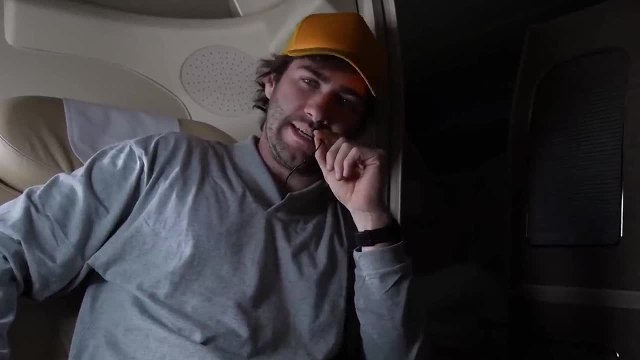 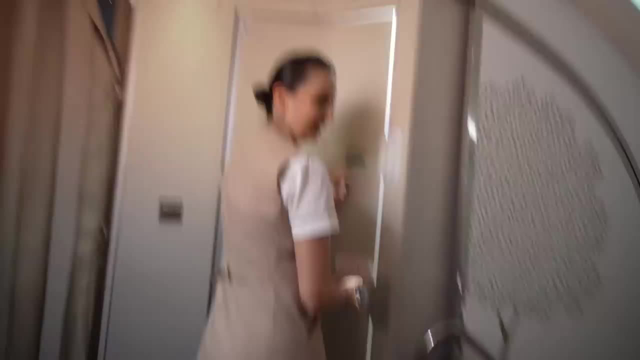 something I've been meaning to do for a long, long time. If I don't do this soon, people might start to hate me. Let's take this to the bathroom. After so many hours on the airplane, it was finally time to experience the main event. 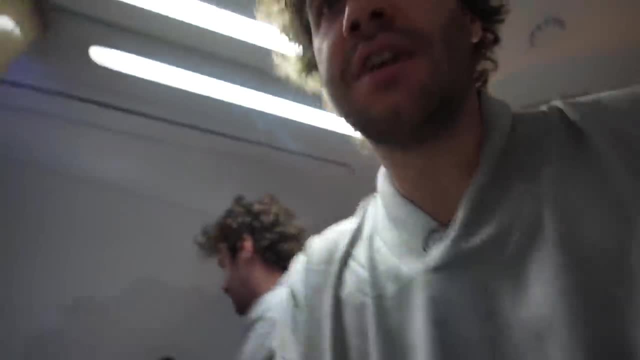 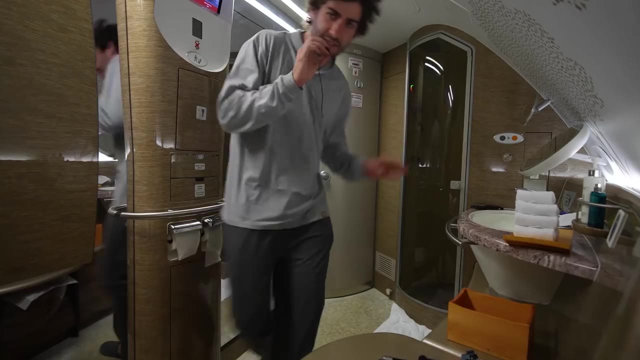 the legendary first class shower and spa. This is the size of my actual bathroom Like this is the size of like a kitchen walk-in closet. She just explained to me that I have five minutes of running water. There's a timer inside of that shower. 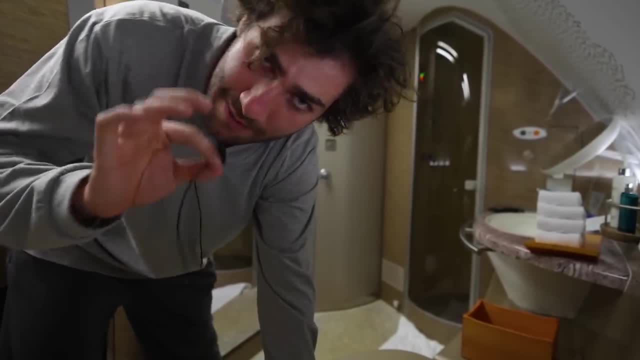 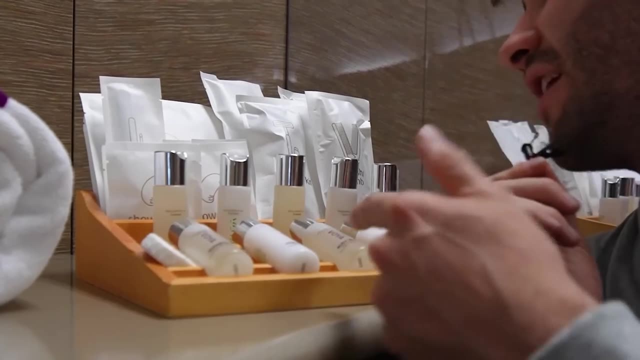 It's like a video game And I basically have that amount of time to wash my body. It makes a lot more sense why they call this a spa. There's a stack of hot towels, an array of shampoos, conditioners, soaps, shaving kits. 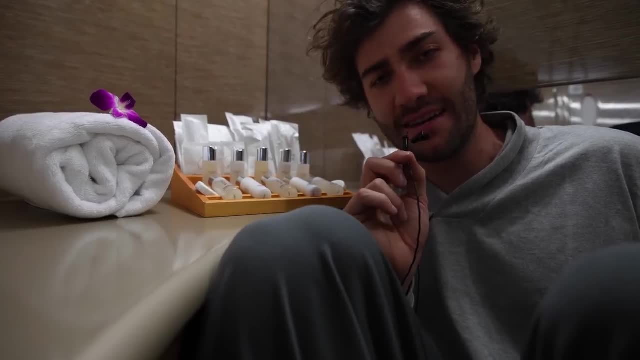 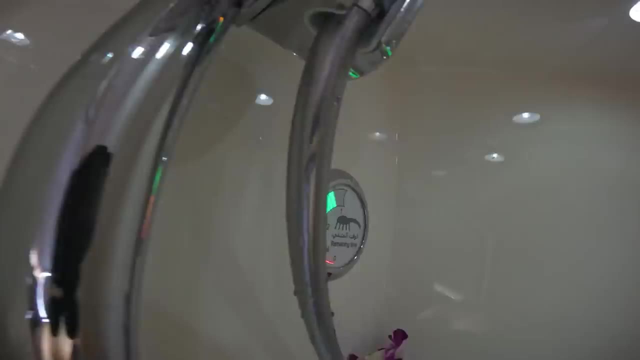 Let me take my shoes off. Oh my gosh, These floors are heated. I guess I'm gonna de-robe. We have five minutes of water on the clock. Okay, here we go. Ah, this is weird. We're slowly running out of water. 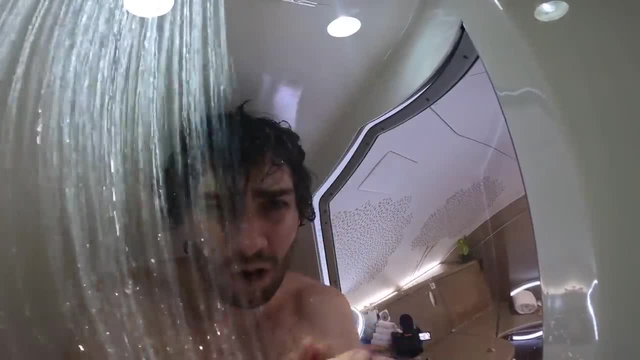 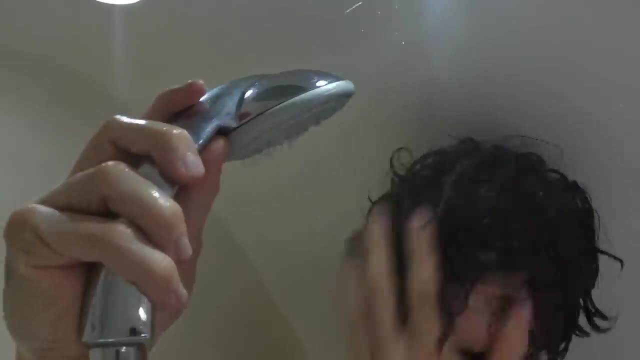 I don't think I'm gonna have time to shampoo. I think I'm only gonna have time to wash my body. I needed this so bad. This might be the most expensive shower I've ever taken. That's it. That was a magical experience. 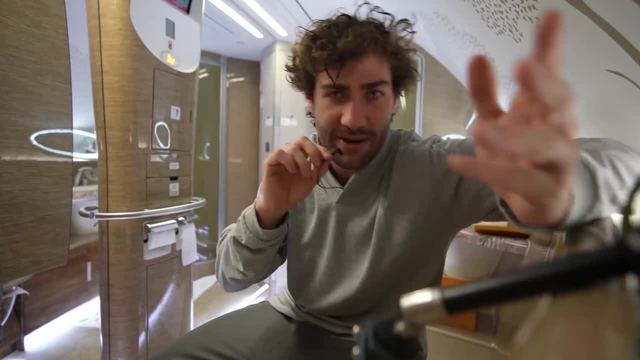 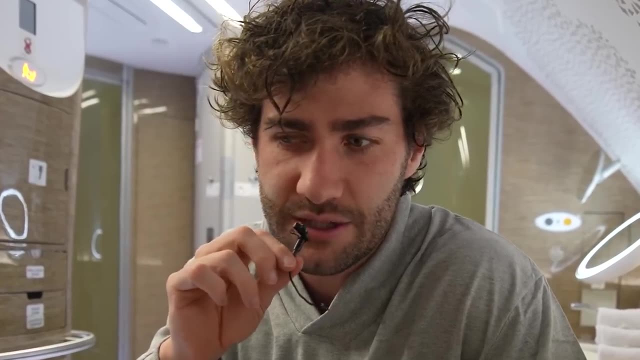 The only thing I really feel like missing is a gym. So, Emirates, if you have like a suggestion box, maybe put a weight room somewhere in here. Adding weight does kind of feel like the opposite of flying, but you guys figured out how to get. 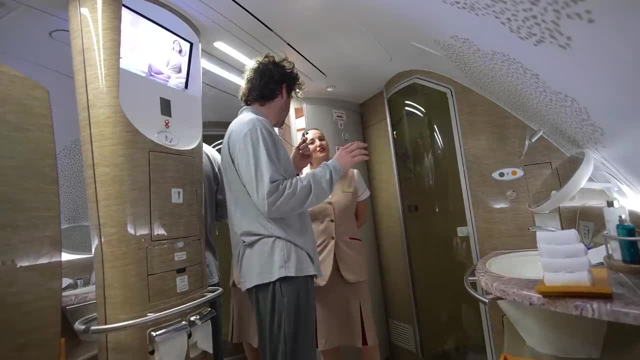 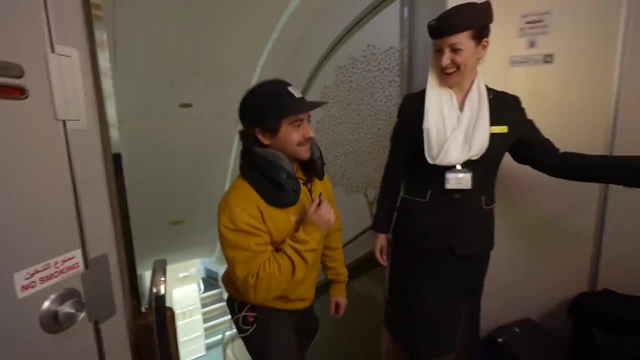 a two-story airplane off the ground, so I trust that you guys can figure this one out. Once I emerged from that unbelievably relaxing shower experience, I decided to ask the flight attendants to bring up a special guest. There he is. Oh my gosh. 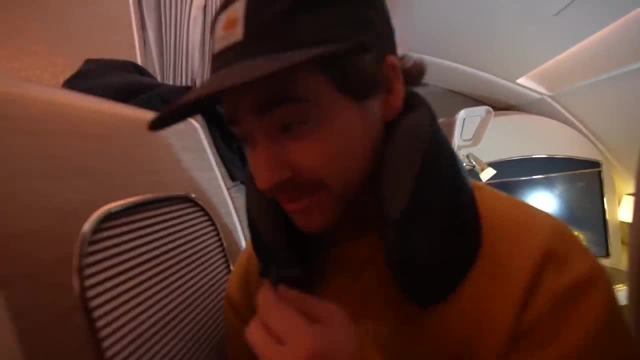 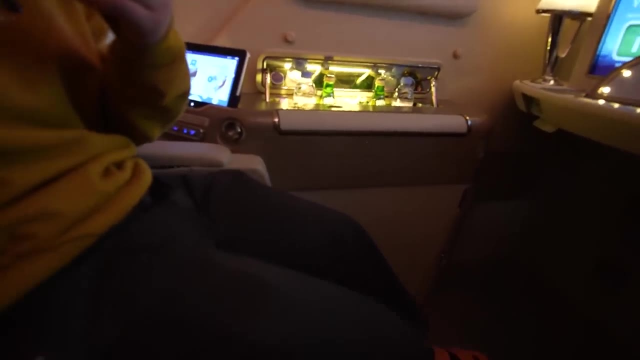 Oh my gosh, Oh dude, I knew you had flat screen TVs. Yeah, just sit down right there. This seatbelt's made of gold, Mine's made of gold. I have the tears of the past passengers, So this is suite 1F. 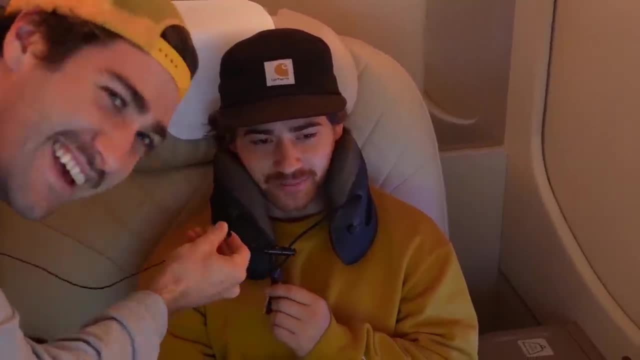 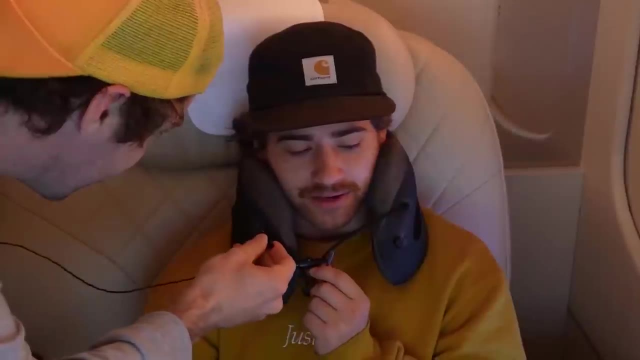 Do you understand the significance of that at all or No, it's a freaking number and a letter. What's so great about 1F? This was supposed to be your suite. This is an empty suite right now. I don't care. 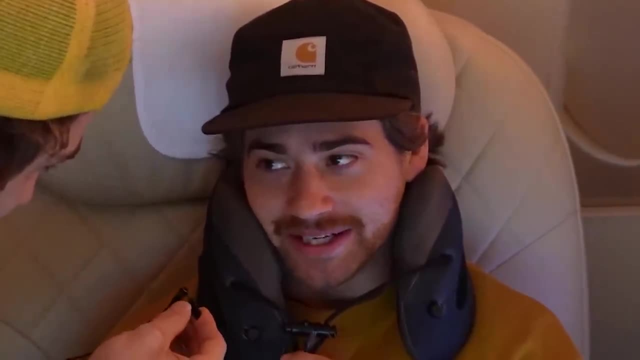 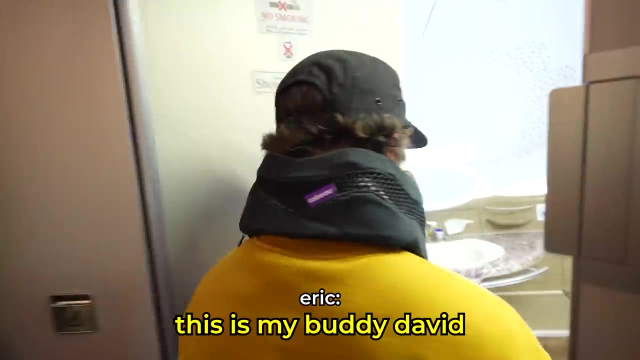 I'm making friends down in Economy. I'm like the mayor of Economy down there. How's the food Delicious Really. What'd you have? freaking luxury cat or something? Whoa, This is my buddy, David. I did make some friends, actually. 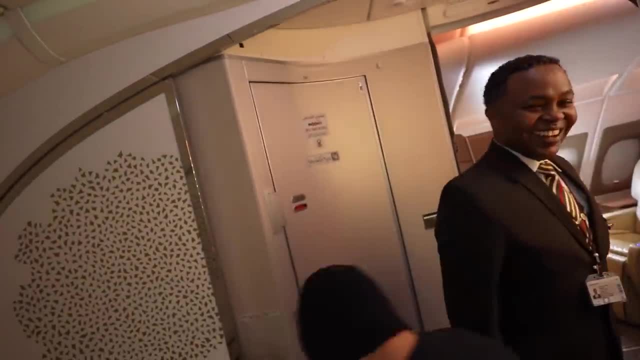 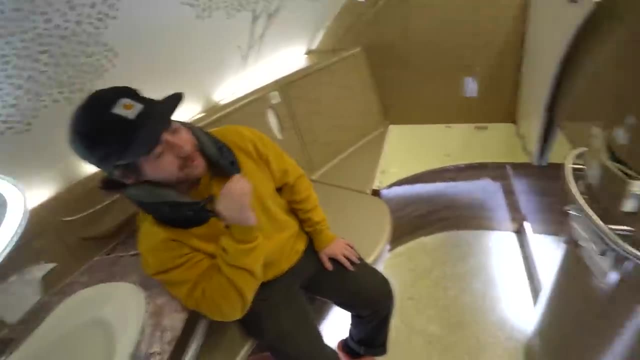 Hey, David, I'm from Economy. You've probably heard of me. He's not heard of you. Wait, is this a bathtub? There's the shower right there. What the You can just sit here and think about how much money you have. 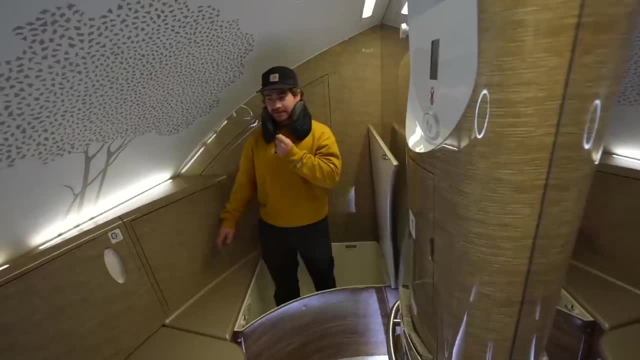 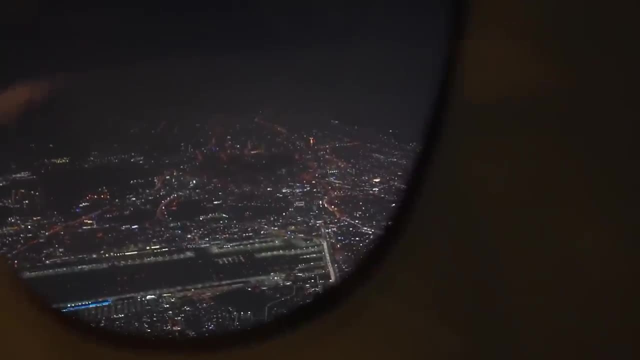 and how lonely you are at the top of the plane. No, no, no, no. Are you ready to get back to Economy? Yeah, I love Economy. By the time Bean's headed back to his seat, we were finally descending towards our destination. 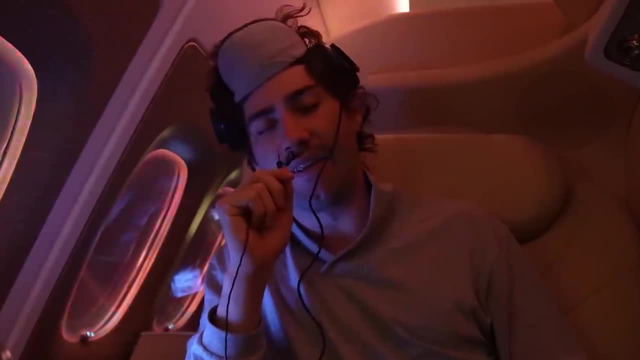 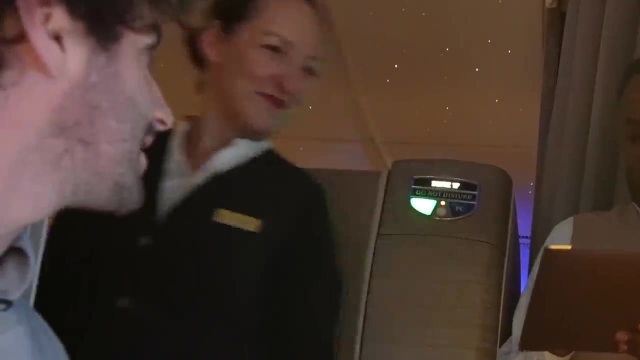 I've had a more luxurious stay inside of this little room than I have ever had on the outside world, And I think, as we descend, it's about time for the review. I'm a little nervous. These crew members took care of every possible need. 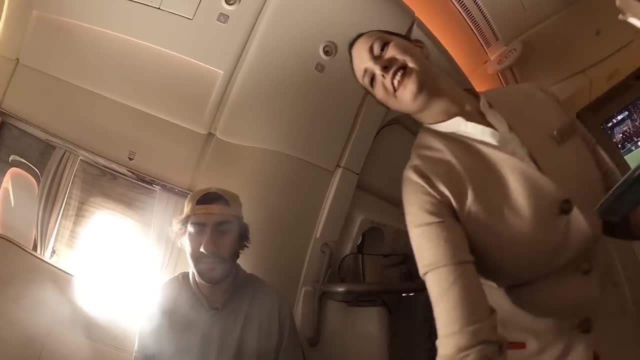 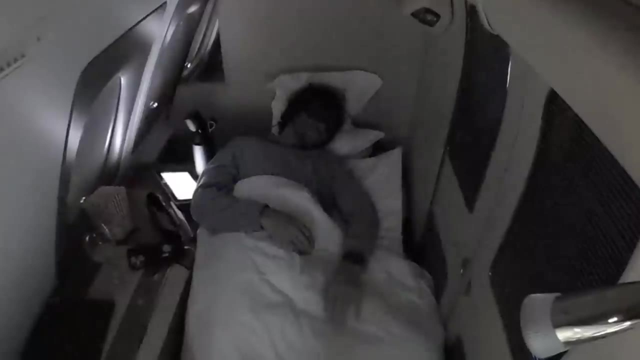 I could have had. And not only that, I set up cameras inside of this airplane the entire time. I was so annoying And they were nice to me. Five out of five stars Comfort. I don't know if I have to really explain myself here. It is the most ridiculous comfortable experience I have ever had on an airplane- Five out of five stars. And lastly, price. I actually did some math on this. If you break down the total cost of the ticket, it was $1,400 per hour or $23 per minute. 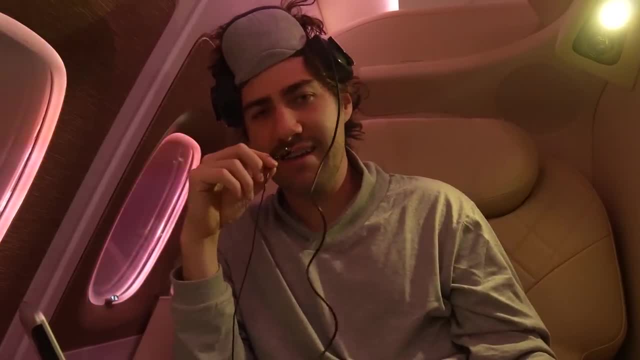 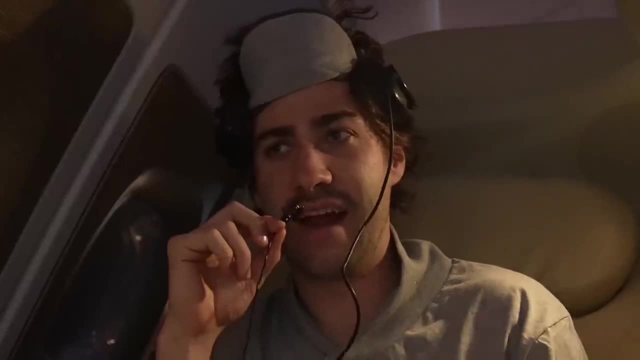 If you get into those terms, there's almost no way to justify it. For the right person, the plane ticket cost probably doesn't even matter, But for me, for us, I feel like this is a little crazy, And for that I have to give price a two out of five stars. 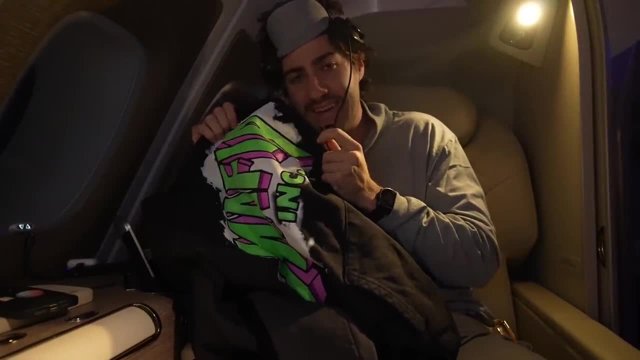 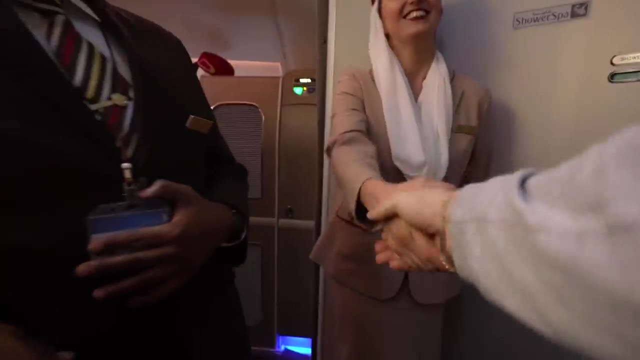 I'm going to have to sell a lot of mafia hoodies to ever sit here again. Please go to airrackshop. These videos are so expensive. And with that the plane finally landed And it was time to give our brutally honest reviews.